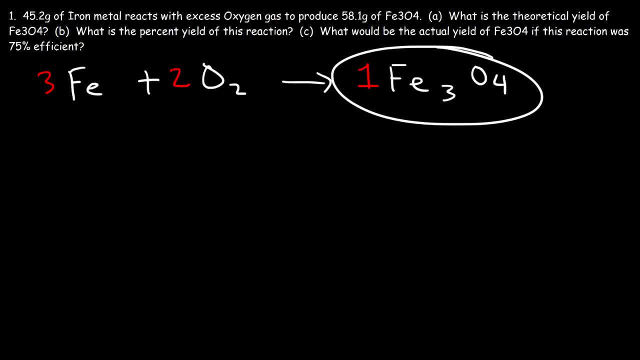 that can be produced in this reaction. That is the theoretical yield. So what we need to do is to convert the grams of Fe. that's the limiting reactant. we need to convert that to the grams of Fe3O4.. O2 is the excess reactant. So now in 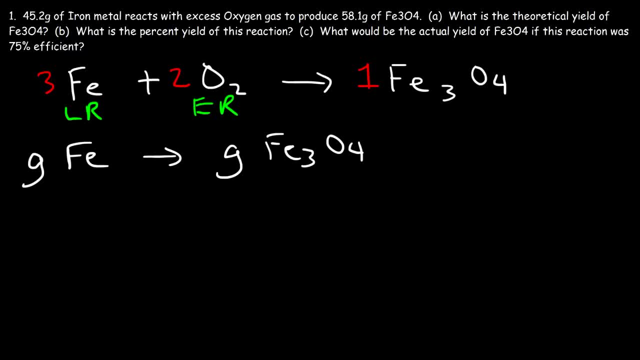 order to convert the grams of one substance into the grams of another substance. it's a three-step process. We're going to start with the grams of Fe and we're going to convert it to the moles of Fe using the molar mass In. 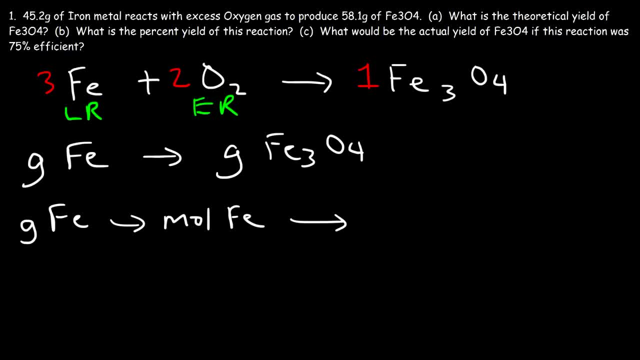 the second step we're going to use the molar ratio to convert from moles of Fe to moles of Fe3O4.. So basically, in the first step we're changing the unit grams to moles. In the second step we're changing the substance from Fe to Fe3O4.. 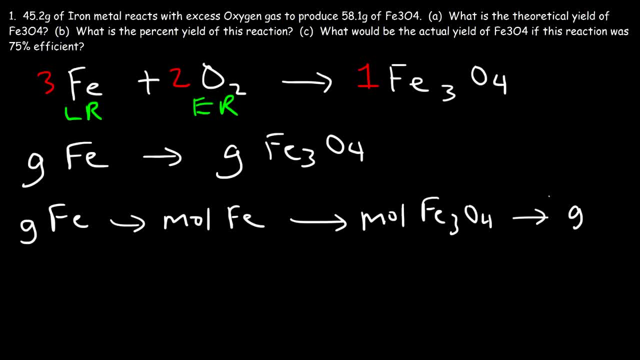 And in the last step we're going to convert to grams of Fe3O4 using the molar mass again. So let's start with what we're given, which is 45.2 grams of Fe. Now the molar mass of Fe is 55.85 grams per mole. So the unit grams of Fe. 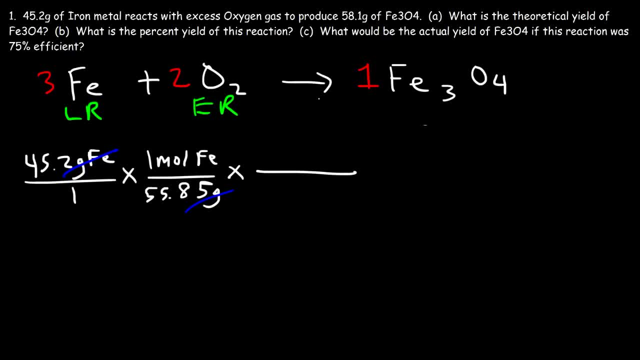 will cancel. And now let's change the substance from Fe to Fe3O4.. So it's a three-to-one ratio. So for every three moles of iron metal that reacts, one mole of Fe3O4 will be produced. So now let's convert this back. 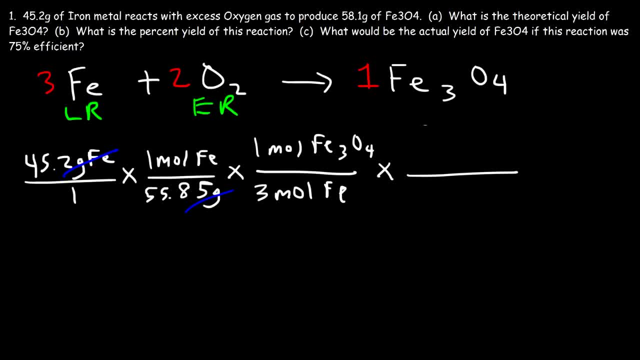 to grams. So we need to find the molar mass of Fe3O4.. So there's three Fe atoms and four oxygen atoms. So it's going to be three times 55.85 plus four times 60. So that's about 231.55 grams per mole, So one mole of iron. 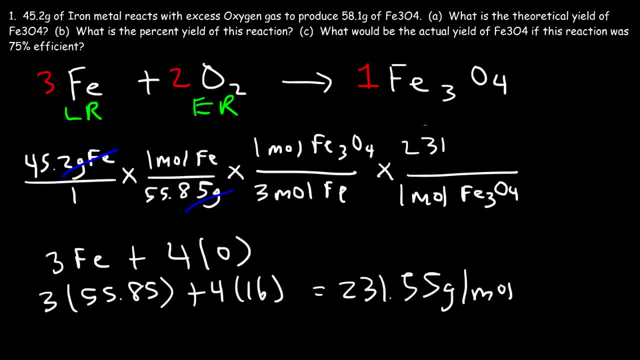 oxide has a mass of 231.55 grams. Always make sure that every other unit cancels, except for the unit that you want, which is grams of Fe3O4.. So now let's perform the operations. It's going to be 45.2 divided by 55.85, divided by three times 231.55.. So this is the 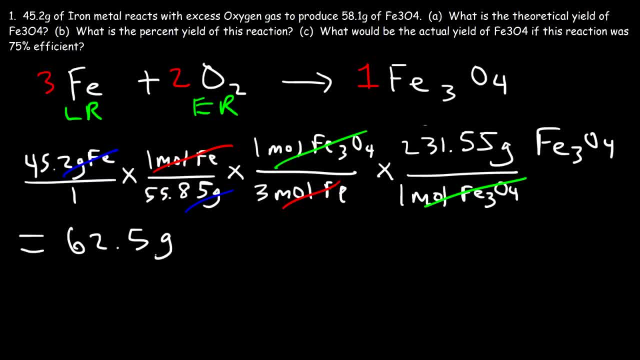 theoretical yield: 62.5 grams per mole. So that is the maximum amount of iron metal- I mean not iron metal but iron oxide- that can be formed in this reaction. You can't get any more than this. So that's the answer to Part A, That's the theoretical yield of Fe3O4.. 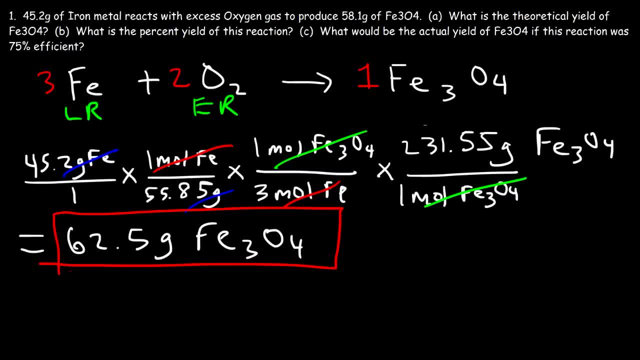 Now let's move on to our next step. How can we find the percent yield of this reaction? The percent yield is equal to the actual yield divided by the theoretical yield times 100%. So we have the theoretical yield and we know its 62.5.. But what is the actual yield? 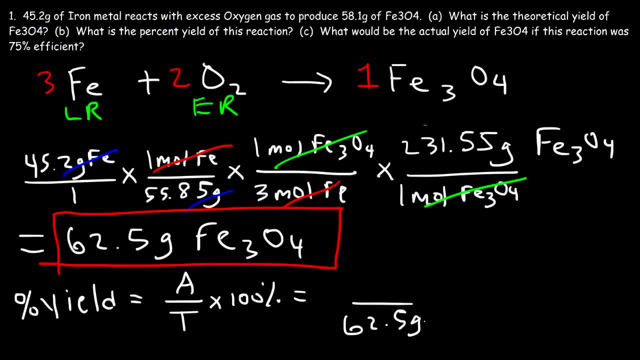 The actual yield is the grams or the moles of the product given to us in the reaction or in the problem. We were given that 58.1 grams of Fe3O4 was actually produced in this reaction, So that is the actual yield. 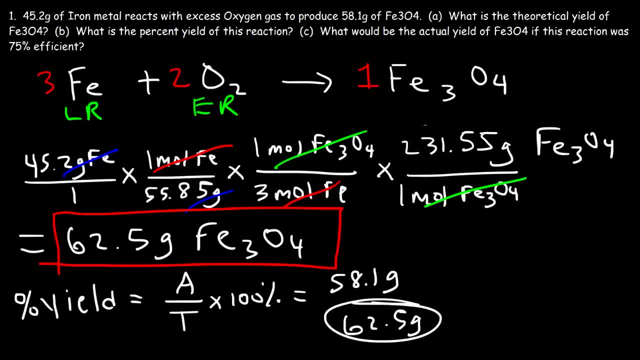 The actual yield should be less than the theoretical yield, it should never be more and it should correspond to the same substance, Fe3O4.. So let's divide 58.1 by 62.5 and then multiply that result by 100.. 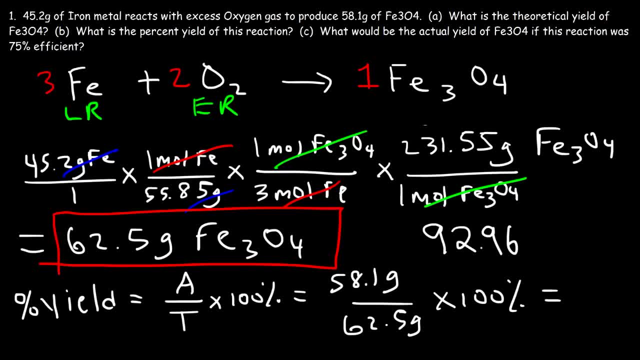 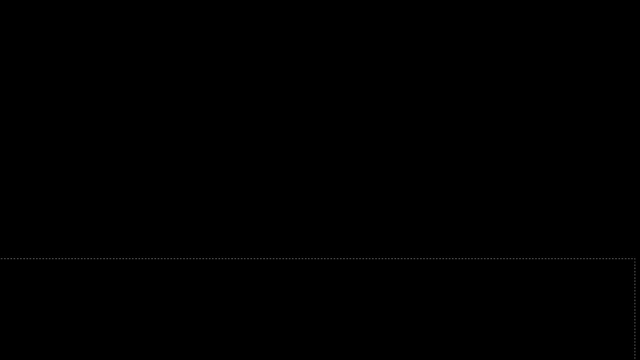 So the percent yield is 92.96, which we could say it's roughly about 93%. So that's the percent yield of this problem. So this particular situation is 93% efficient. Now let's move on to part C. Okay, I didn't want everything to be deleted. 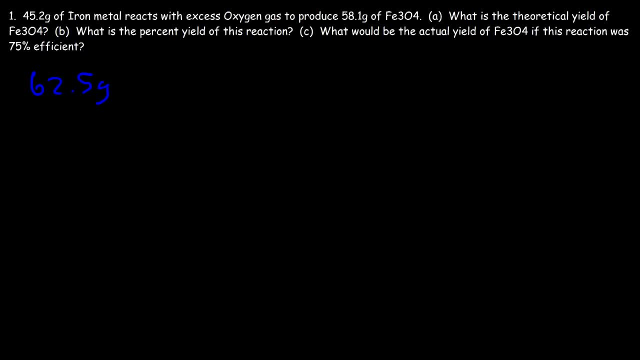 Now keep in mind the theoretical yield is still 62.5 grams. We're going to need that value. Part C: Let's see what would be the actual yield of Fe3O4 if this reaction was 75% efficient. If the process was 100% efficient, the actual yield would be the same as the theoretical. 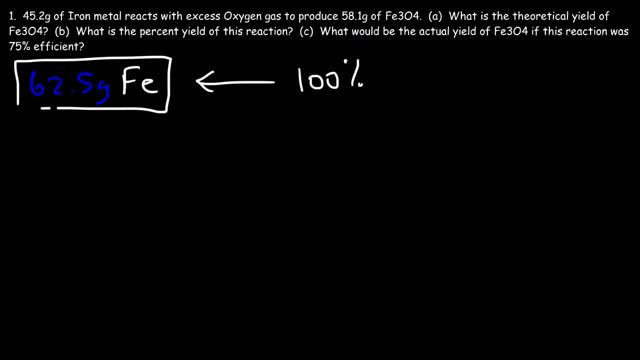 yield. So the theoretical yield is 62.5.. If it was 100% efficient, that's how much product we would get in the reaction, And it's supposed to be Fe3O4.. I don't know why I keep writing it as Fe. 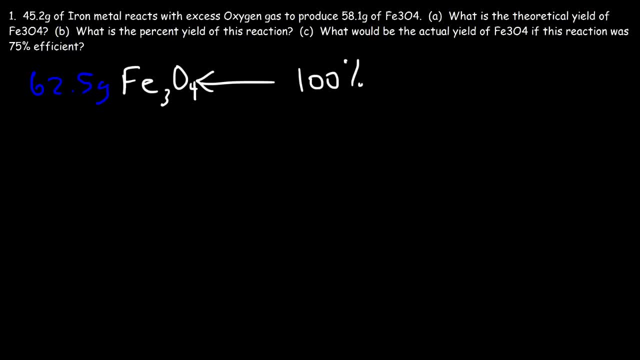 So if it's 75% efficient, that means in the course of the reaction we should get 75% of the theoretical yield. So all we got to do is multiply 62.5 by 75%. The decimal equivalent of that is 0.75.. 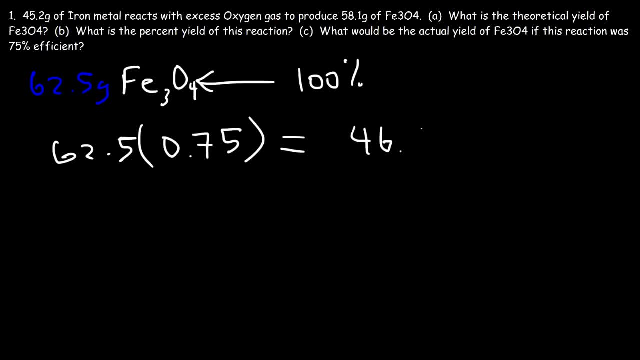 So if it was 75% efficient, the actual yield will be 46.9 grams of iron oxide. Okay, Let's see Now. granted, you can use the equation to get the answer as well. You could say: percent yield is equal to the actual yield divided by the theoretical times. 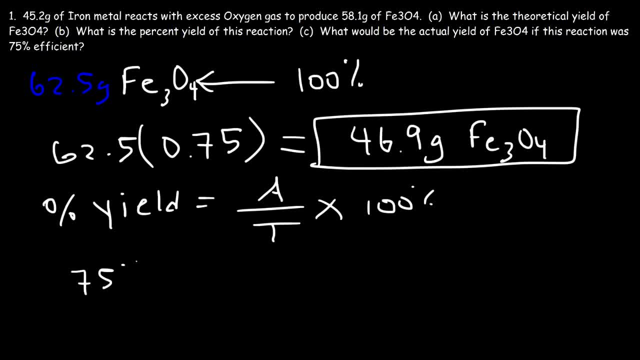 100. So the percent yield is 75%. You're looking for the actual yield. The theoretical yield is 62.5 times 100. So first you would have to divide both sides by 100. So 75% divided by 100 would give you 0.75. 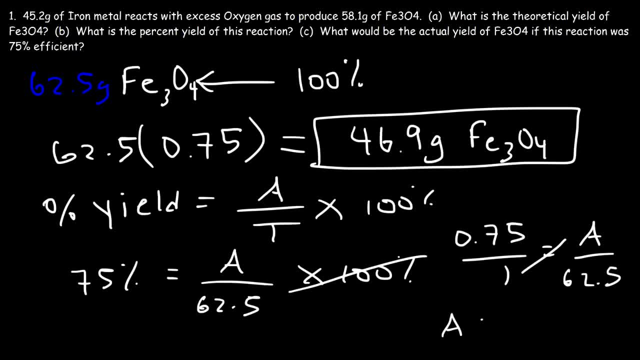 And then you would have to cross-multiply One times. A is A, and that's equal to 0.75 times 62.5, which is 46.9.. So all you need to do is just multiply the theoretical yield by the decimal equivalent. 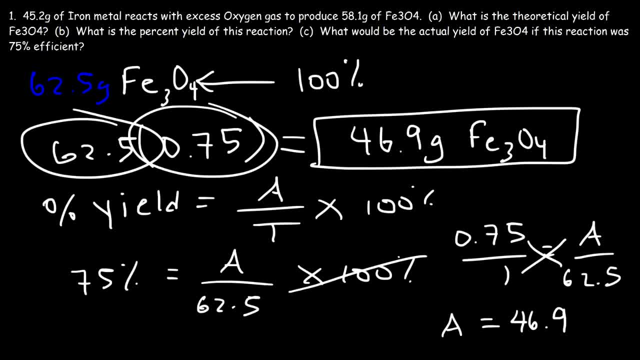 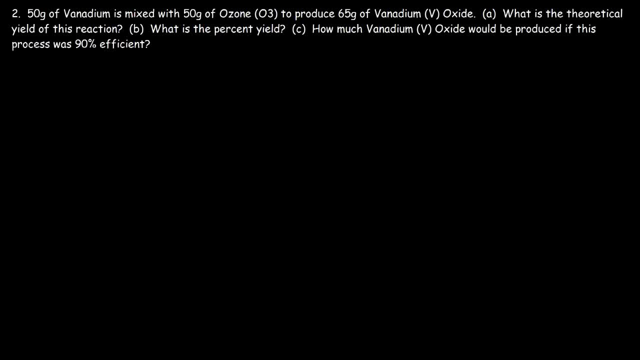 of the percentage and that's going to give you the actual yield. Go ahead and try this one. It's a similar problem to the last example: 50 grams of vanadium is mixed with 50 grams of ozone to produce 65%. 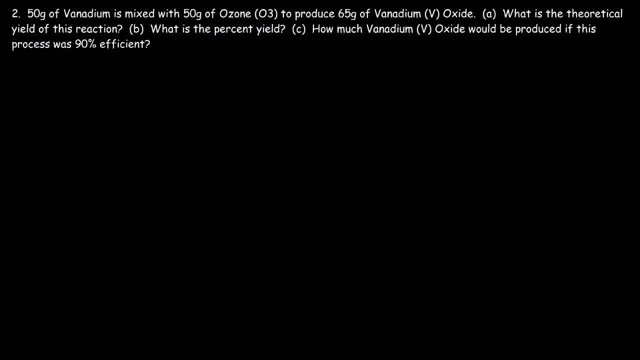 What is the theoretical yield of this reaction? So let's write a balanced equation: Vanadium is V, Ozone is O3, and we need to find the chemical formula of vanadium oxide. So the Roman numeral 5 tells us to charge on vanadium. 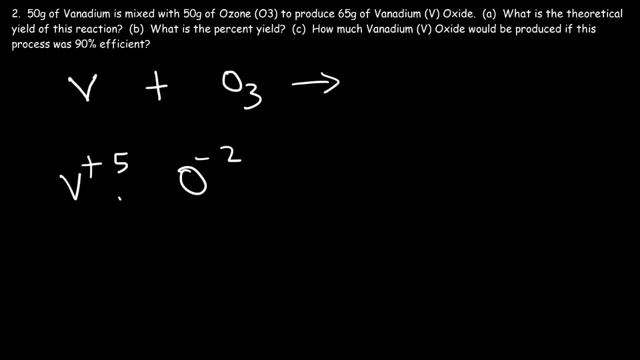 It's positive 5.. Oxygen has a negative 2 charge as an ion, So this is going to be V2O5.. So now we need to balance the equation. In order to balance the number of oxygen atoms, find the least common multiple between 3 and. 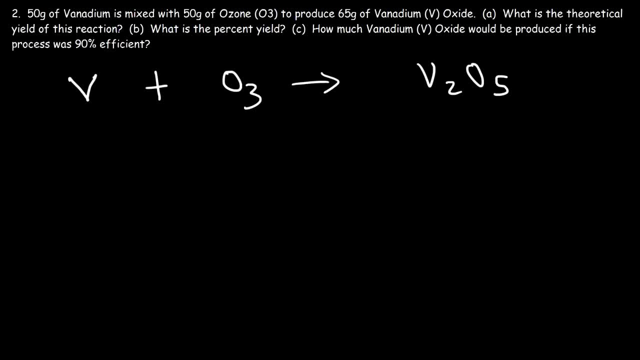 5.. 3 times 5 is 15.. So we need 15 oxygen atoms on both sides. So let's put a 5 in front of O3, and a 3 in front of V2O5.. Now we have 6 vanadium atoms on the left, so we need to put a 6 in front of V. Now this: 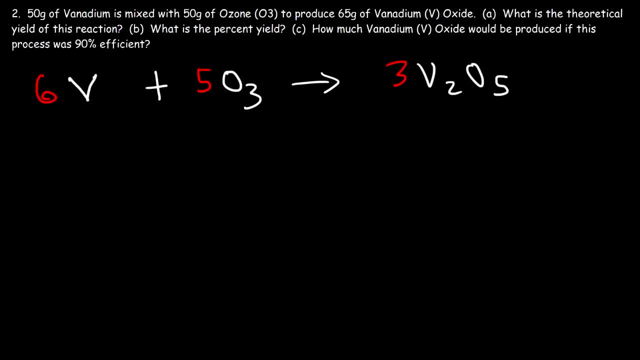 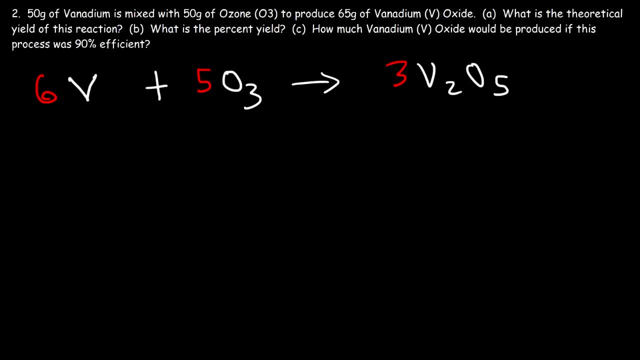 We knew which reactant was limited and which one was excess. In this example, we don't know. So what I'm going to do is I'm going to convert the grams of each reactant to the grams of product, which is vanadium oxide. 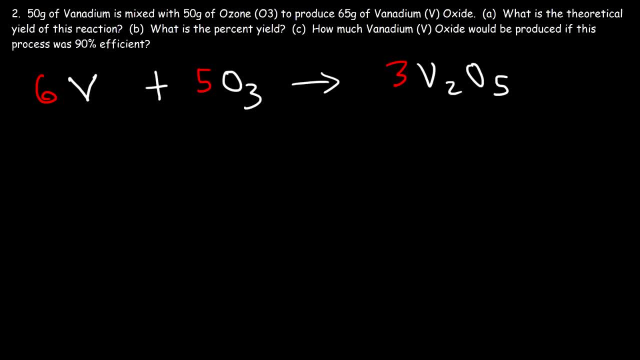 The limited reactant will give us a lower theoretical yield. Whichever number is less, that's going to be the actual theoretical yield, and the reactant that gave us that answer is the limited reactant. So let's start with 50 grams of vanadium. 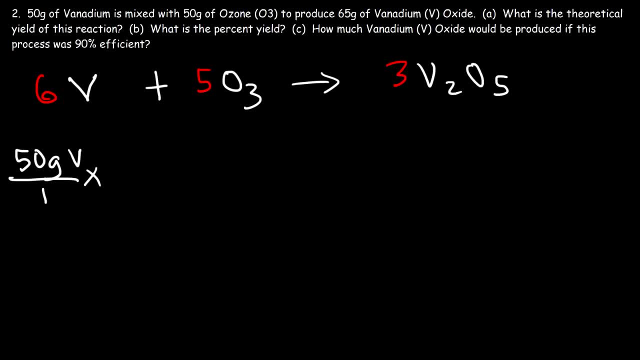 Let's convert it to moles. The molar mass of vanadium is 50.95, I mean, excuse me, 50.94 grams per mole. So one mole of vanadium is equivalent to 50.94 grams. Now we need to convert from 50.94 grams to 50.94 grams per mole. 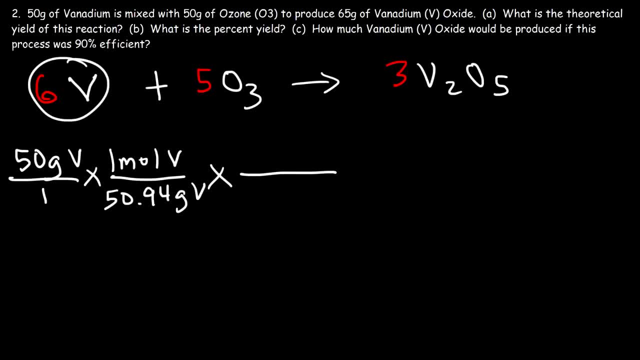 Moles of vanadium to moles of the product vanadium oxide. The molar ratio is 6 to 3.. So for every 6 moles of vanadium that reacts, 3 moles of vanadium oxide will be produced. 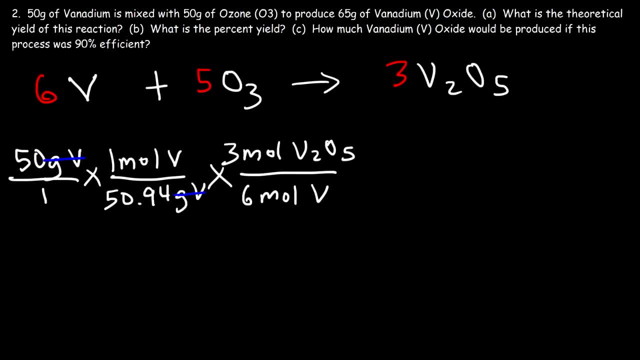 So we can cancel the unit grams of vanadium and moles of vanadium. Now we need to find the molar mass of vanadium oxide. So there are 2 vanadium atoms in that compound and 5 oxygen atoms. So we need to find the molar mass of vanadium oxide. 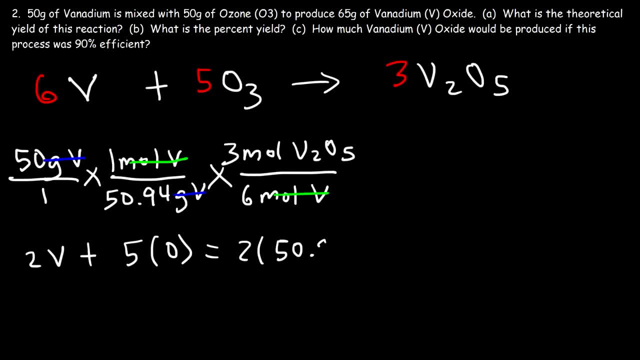 So there are 2 vanadium atoms in that compound and 5 oxygen atoms. So this is going to be 2 times 50.94 plus 5 times 16.. Five times 16 is 80, and 2 times 50.94, that's 101.88.. 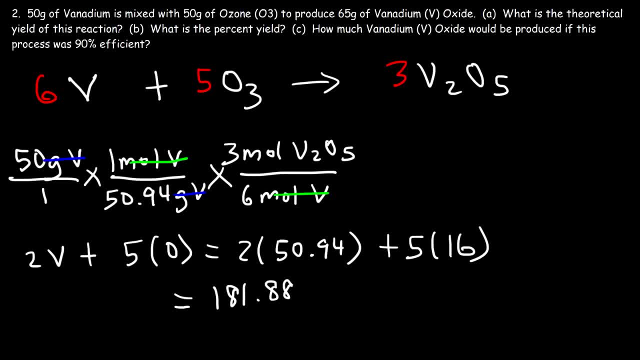 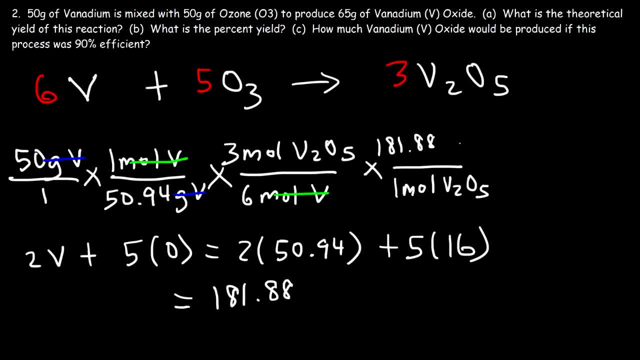 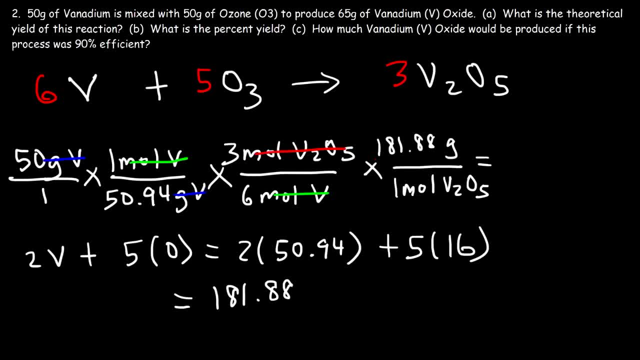 So one mole of V2O5 has a mass of 181.88.. So one mole of V2O5 has a mass of 181.88.. So automatically we're getting a mixture of 30, who created 6 moles of vanadium. 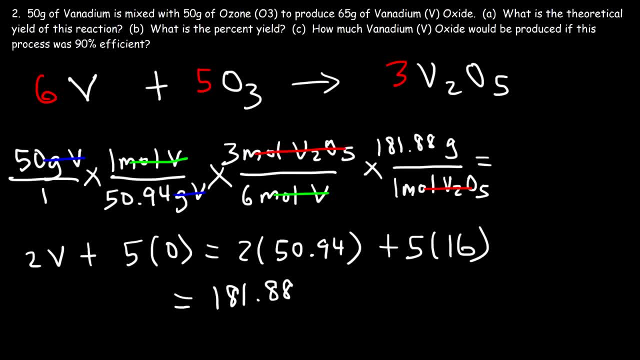 plus 1 mole of V2O5.. Alright, good work. everyone. Have a great afternoon. See you at school, Peace out. Thanks for watching. Now you need to understand what this number means. It may or may not be the theoretical yield. 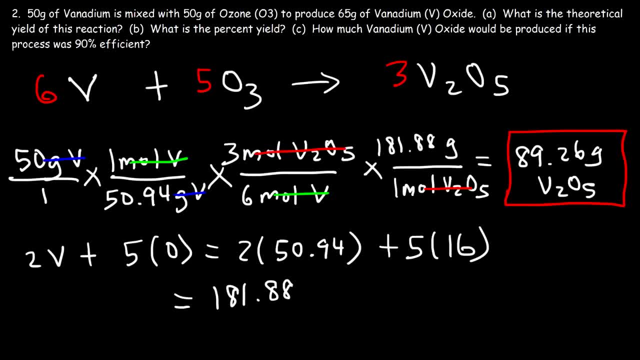 We don't know yet. All we know is that if all of the 50 grams of vanadium reacts, if it's the liminary reactant, then 89.26 grams of V2O5 will be produced. But we don't know if V is the liminary reactant yet. 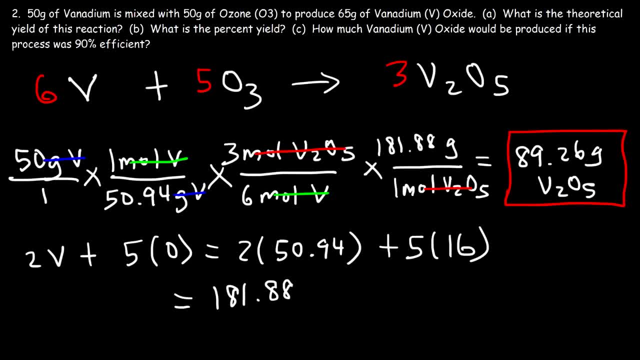 But we're about to find out soon. Now let's start with the other substance: 50 grams of ozone, And let's convert it to moles. The molar mass of O3 is 16 times 3,, which is 48.. 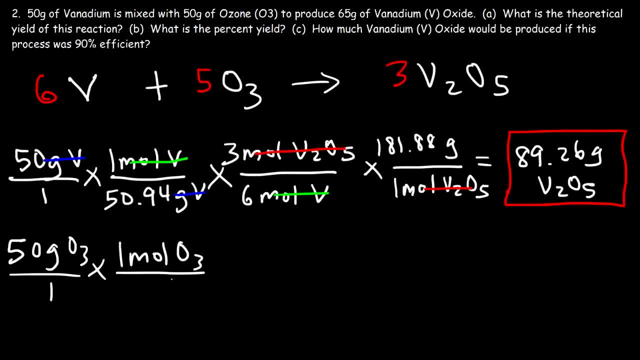 So one mole of O3 has a mass of 48 grams. Now let's convert from O3 to V2O5.. For every 3 moles of V2O5 that's produced, 5 moles of O3 will react. 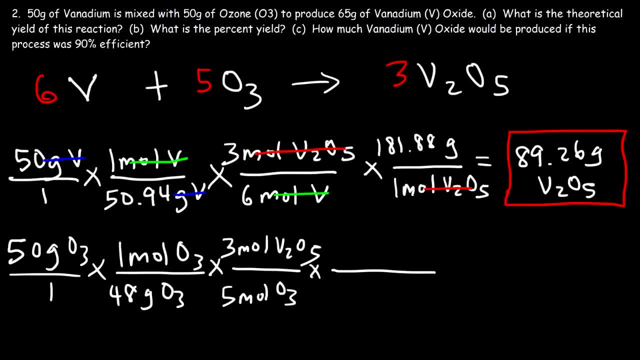 Now the last part is going to be the same. The molar mass of V2O5 is 181.88 grams. So, as you can see, whenever you're doing a gram-to-gram conversion, the setup is still the same. 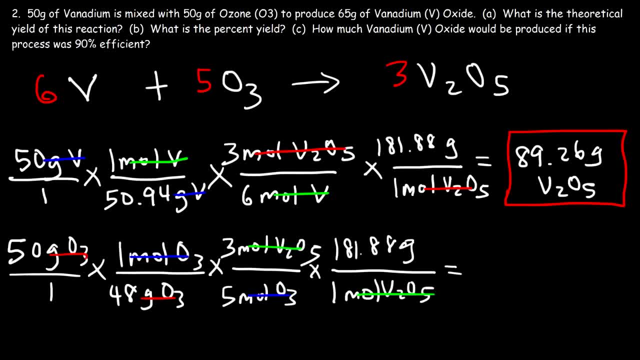 So this is going to be 50 divided by 48, times 3, divided by 5, times 181.88.. So if all 50 grams of ozone reacts, 113.675 grams of vanadium oxide will be produced. 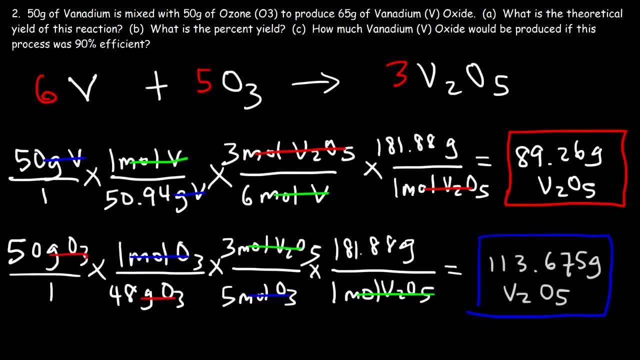 So therefore, looking at these two numbers, which one is the correct theoretical solution? The correct one is the lower number. It's this one, And the reactant that gave us that answer is the limited reactant. So vanadium is the limited reactant. 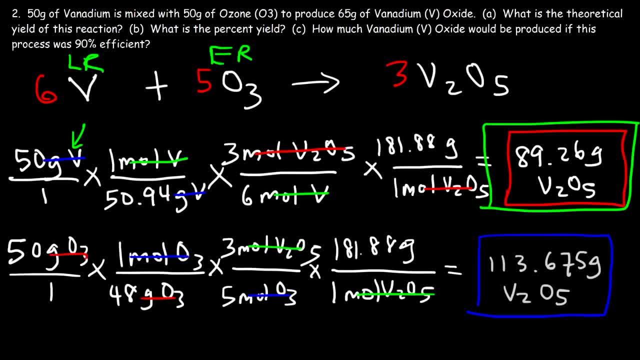 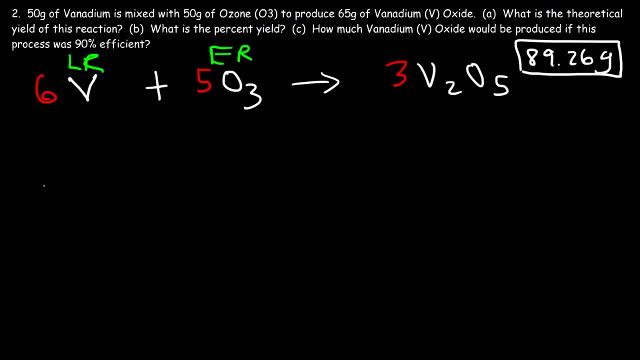 Ozone is the excess reactant. So the answer to part A is 89.26 grams. That is the theoretical yield. Now let's move on to the next part. What is the percent yield? The percent yield is equal to the actual yield divided by the theoretical yield times 100%. 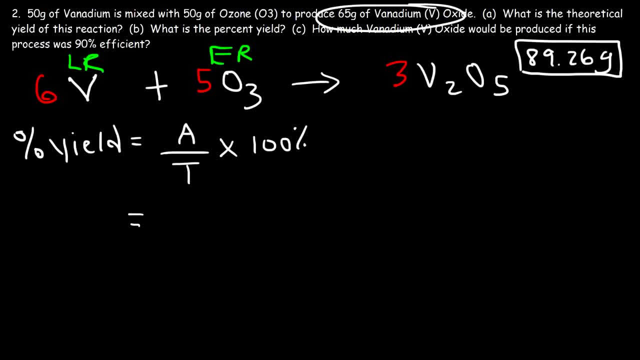 In our example, the actual yield is 65 grams of vanadium oxide. That's how much was formed in this reaction, The theoretical yield. This is the most that we can produce in a reaction If we have a process that's 100% efficient. 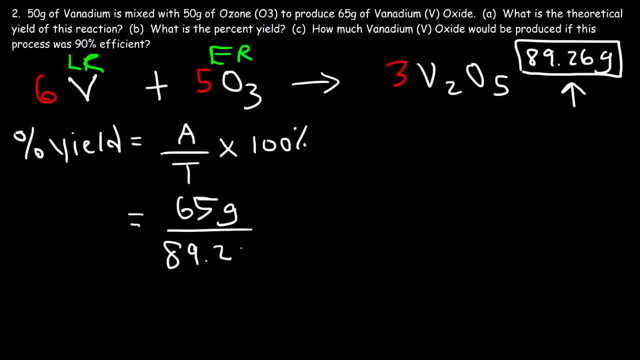 So the maximum vanadium oxide that we can produce is 89.26 grams, But we only got 65 in this experiment. So 65 divided by 89.26, times 100%, That means that this process was 72.8% efficient. 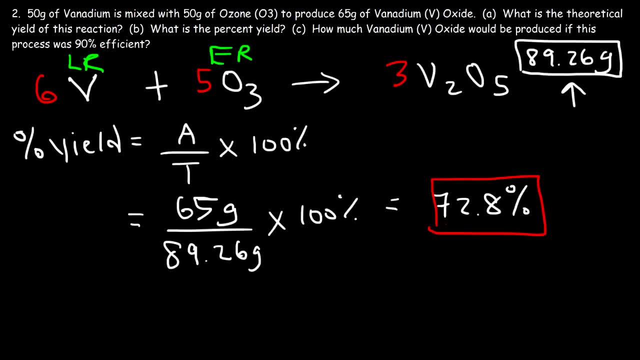 So we only got 72.8% of how much we could have gotten. So we only got 72.8% of how much we could have gotten In terms of the amount of vanadium oxide that was collected. Part C: